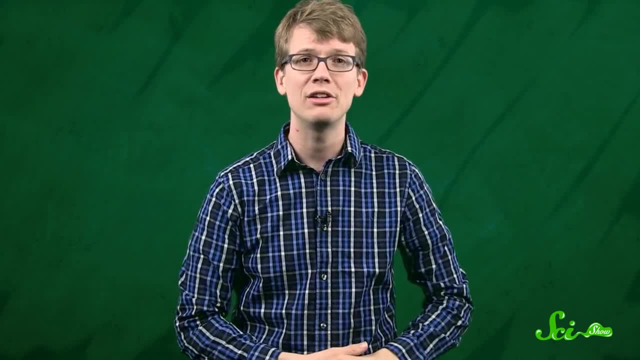 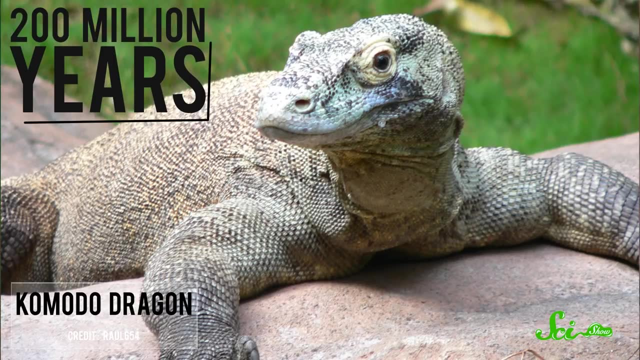 the oldest venomous land lineage And venomous snakes share a common ancestor with venomous lizards like the Gila monster and the Komodo dragon, whose toxic ways go back some 200 million years. Venoms didn't just come out of nowhere. They all evolved through the mutation of protein. 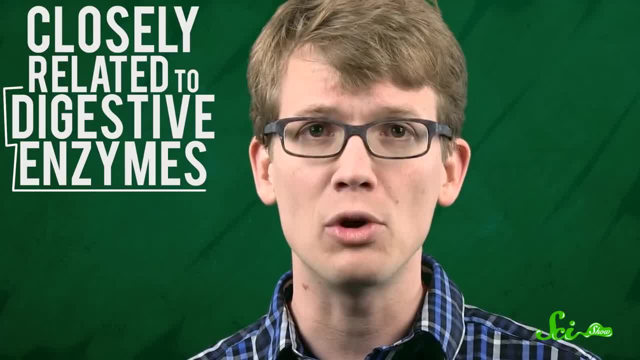 genes. Some venoms are closely related to digestive enzymes, like those found in saliva, while others are more similar to immune system proteins designed to fight off invading bacteria. Although there are low levels of venom in the venomous snakes, some of them are more. 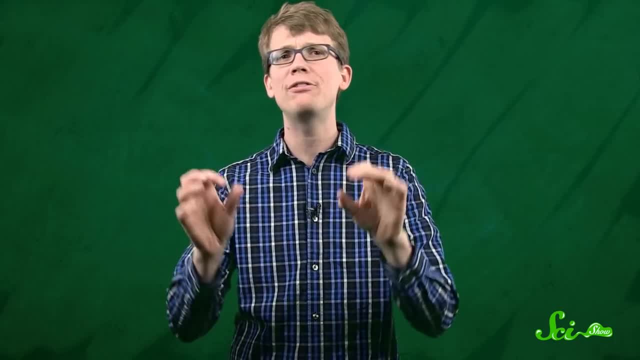 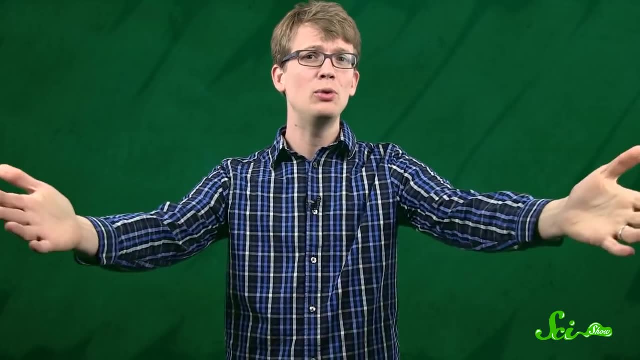 common than others. In addition to the fact that there are loads of different venoms in all sorts of crazy animals, they seem to mostly fall into two broad categories: Those that attack neuron receptors and those that mess with the blood's ability to clot. These are the two best ways. 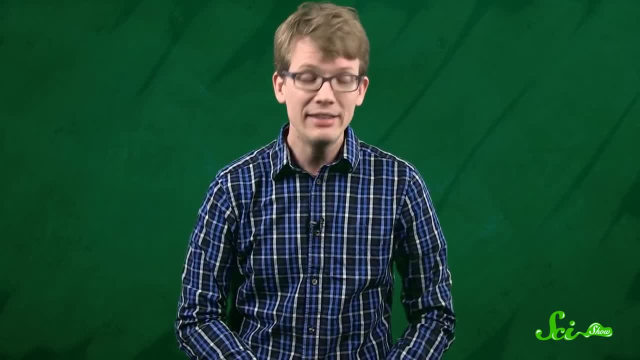 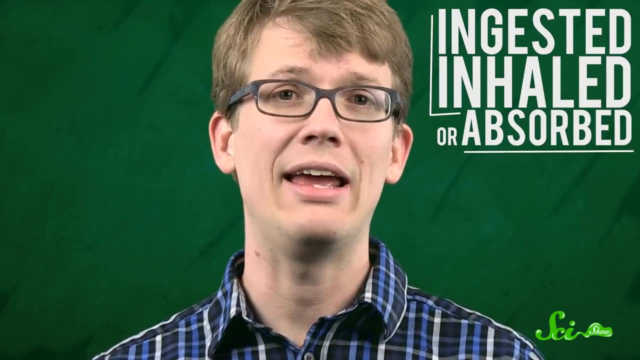 to chemically kill something quickly, Which is why all venoms are similar. whether you're an octopus or an ant, Yes, there are venomous octopuses. Venom is technically different from poison. Poison must be ingested, inhaled or absorbed. 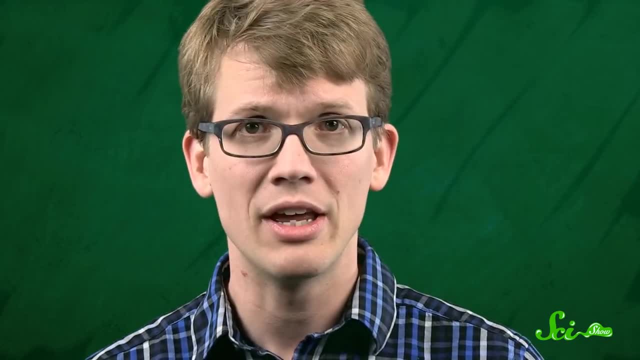 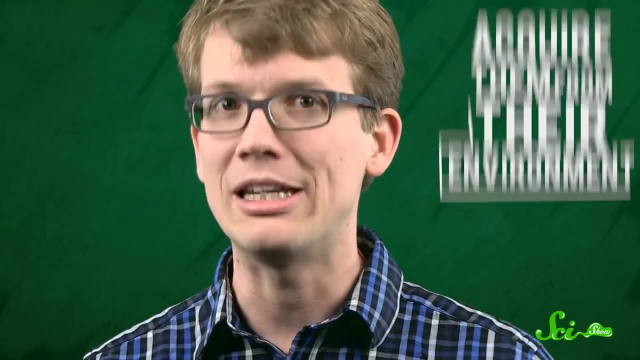 whereas venom is always injected, beaks, tails or tentacles- Venomous creatures brew their own toxins, while some poisonous creatures acquire them from the environment, which is something I'll get back to in a minute. Now it's time to discuss who the biggest, baddest, most deadly toxic avenger of the animal kingdom is? Well, the answer is that we really can't say for sure. There are just too many variables in species, behavior and physiology and environment to say authoritatively who is the deadliest of them all. But we do know that certain animals have acquired the 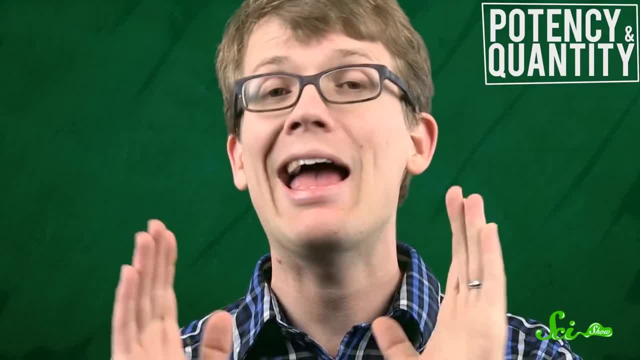 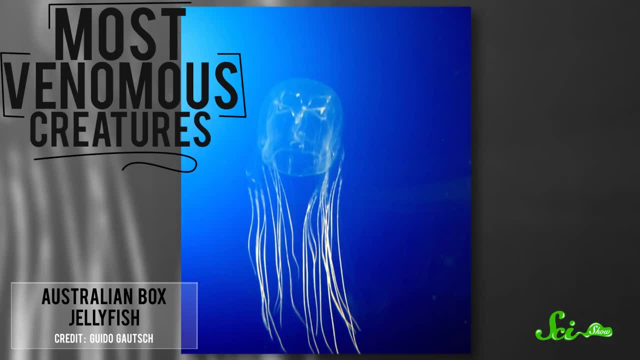 most devastating combination of toxic potency and quantity of poison delivered in a single strike. The Australian box jellyfish, for example, is no doubt one of the most venomous creatures on Earth. This ancient bad Larry has a body the size of a beach ball that trails. 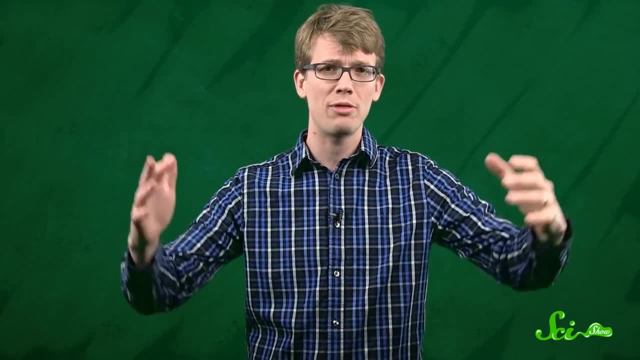 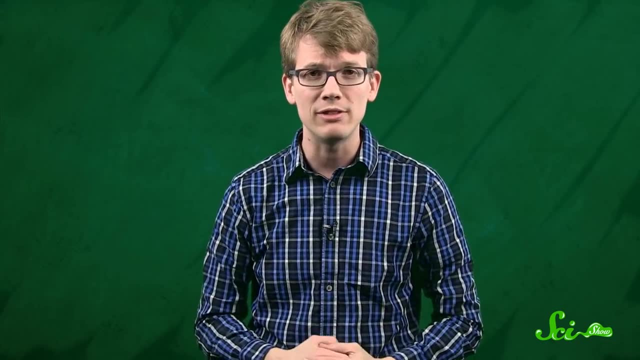 about sixty thin, three-meter-long tentacles, each equipped with millions of nematocysts, harpoon-like mechanisms that spring on contact, injecting venom into its victims. Those little things are a pretty amazing adaptation. After all, if you're a gelatinous blob laughing. both tooth and claw. you can't just blob your prey to death at risk to your own fragile jelly body. You have to totally immobilize it before it can struggle. And the venom that the box jellies carry is one of the most powerful concoctions known A cocktail of neurotoxins. 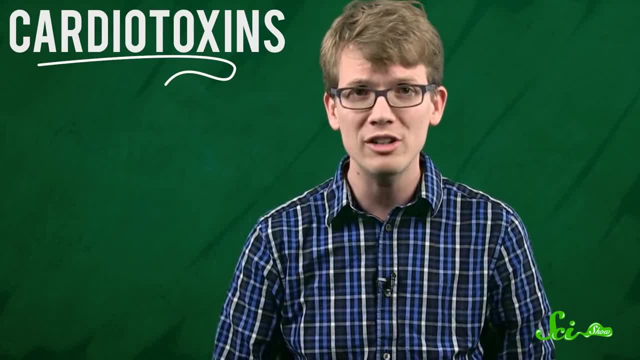 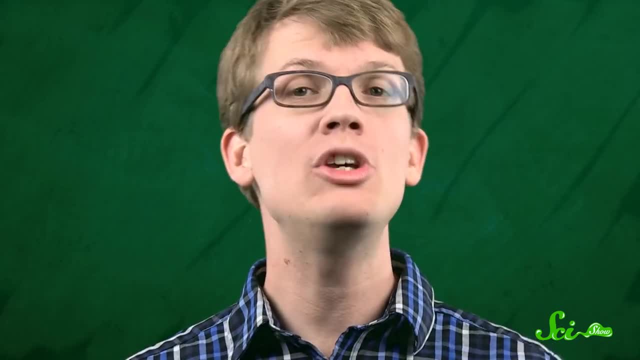 which mess with the nervous systems, cardiotoxins, which try to shut down your heart, and dermonecrotic chemicals that kill living flesh- Just rotting zombie flesh. When a swimming human is unfortunate enough to be stung by one of these blobs, the venom can cause respiratory failure and 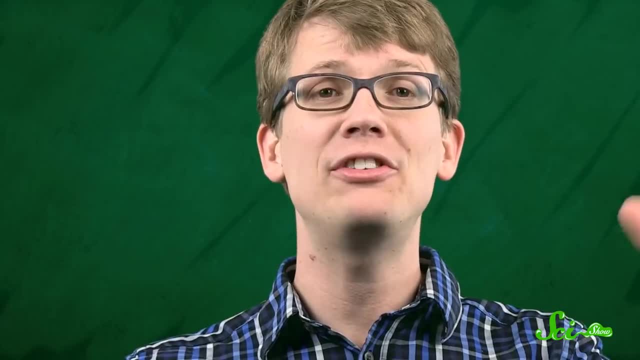 cardiac arrest, And if you're a jellyfish you can't do anything about it. You have to get back a rest- Two things you don't want to have happen to you. In fact, the stings are so intensely and immediately painful that victims often go into shock and drown before. they even ever reach shore. And while you're avoiding beach balls that you're not familiar with at the beach, don't be picking up pretty shells willy-nilly either. Cone snails, found in warm waters all over the world, have extraordinarily long venom glands like tiny transparent harpoons that. 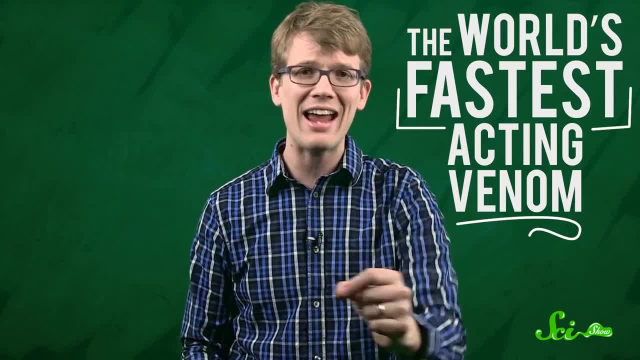 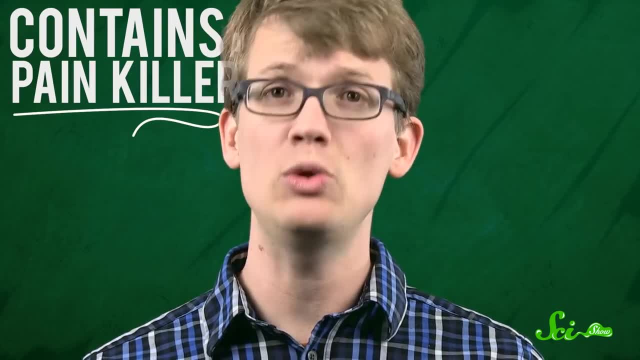 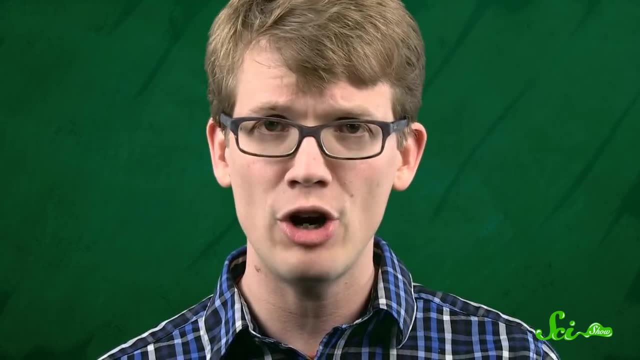 can pierce a wetsuit and inject you with the world's fastest acting venom, which you may not actually even feel. Most venomous creatures produce one or just a few toxins, but the cone snail has up to one hundred different toxins in its arsenal, each designed to target different parts of 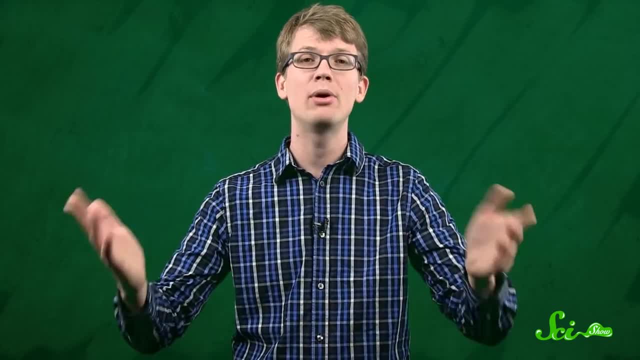 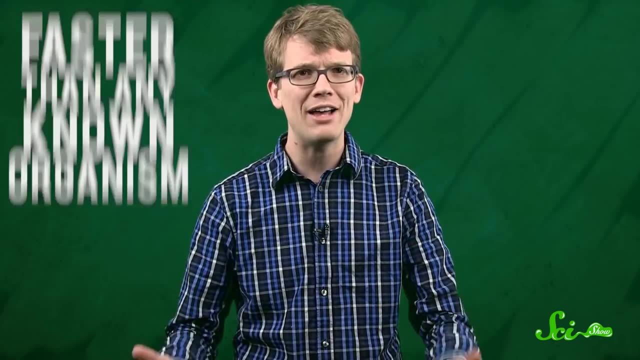 the nervous system. For example, tests on lab mice have shown that one component causes tremors in mice while another puts them to sleep. It's possible that cone snails can produce so many different types of toxins because they duplicate their genes faster than any known organism in the animal kingdom. 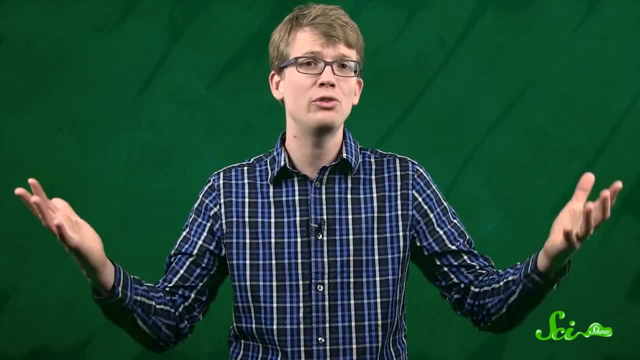 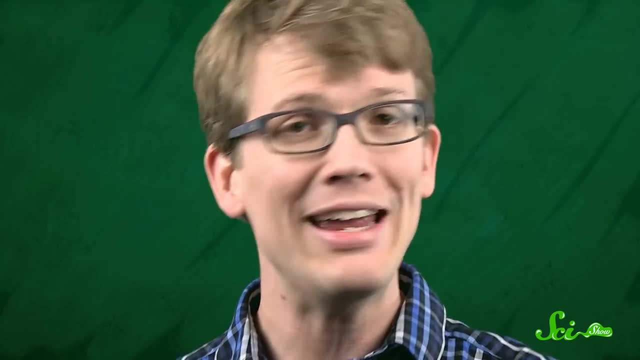 This fast and continuous turnover of their venom genes basically throws their defense mechanisms into evolutionary overdrive. So now you're thinking to yourself: well, I'll just avoid the ocean completely and I'll be safe, right? Well, think again. Over one hundred thousand people worldwide die each. 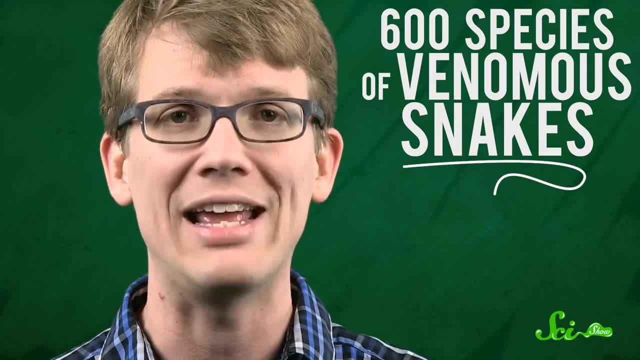 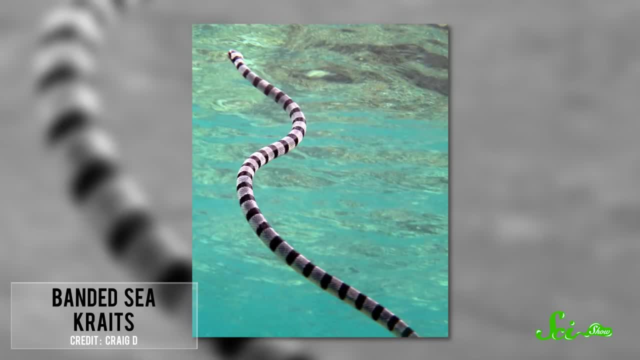 year due to bites from one of the more than six hundred species of venomous snakes on Earth. Snakes prove that having the most powerful toxin doesn't always make you the most dangerous. For example, banded sea crates found in tropical Indo-Pacific waters have incredibly potent. 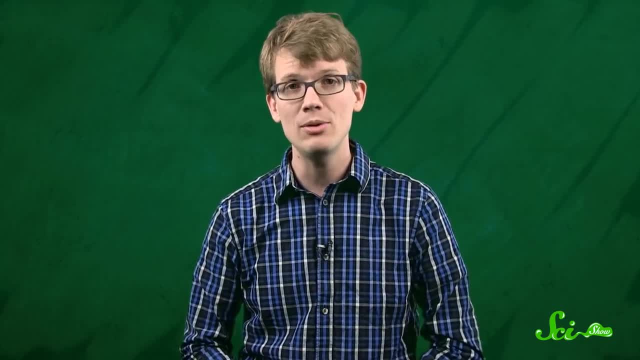 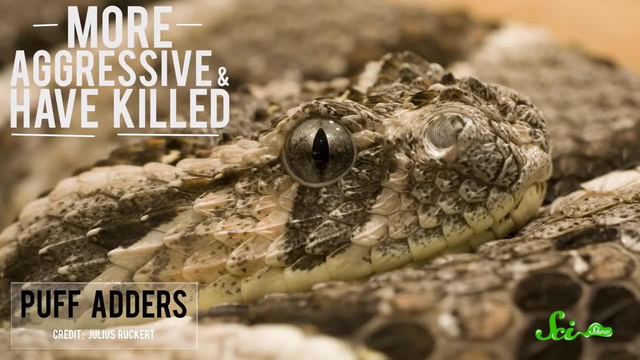 venom, but they're shy and docile and not likely to attack humans, Whereas, if you're curious, puff adders. vipers found throughout sub-Saharan Africa have weaker venom but are more aggressive and have killed lots and lots and lots of humans. King cobras found in Southeast Asia are the world's longest venomous snake, reaching lengths up to nearly six meters. It's terrifying And can unleash enough venom in a single bite to bring down an adult elephant in a few hours. Why? Why do you have that much venom? What? are you going to do with an elephant? And yet the king cobra's venom pales in comparison to that of the Australian inland taipan, Largely recognized as the most venomous snake on the planet. their venom is loaded with typhoxin. 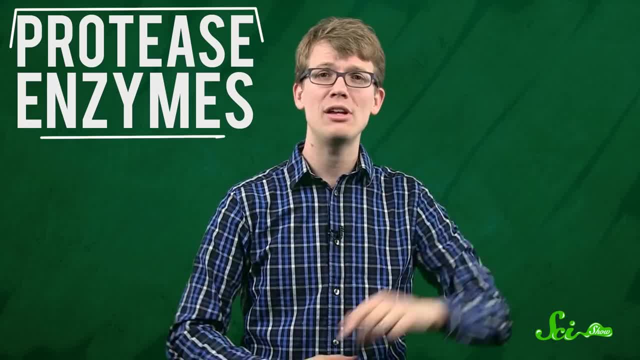 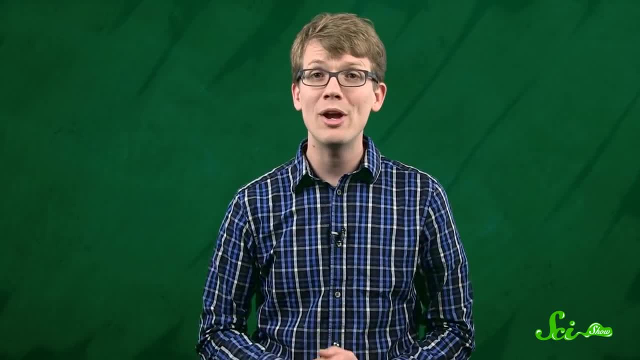 the most lethal known serpentine neurotoxin, along with a dash of protease enzymes to help digest proteins and procoagulants which interfere with blood clotting. But while the inland taipan's venom is record-breaking, it's a shy snake and nearly all recorded. 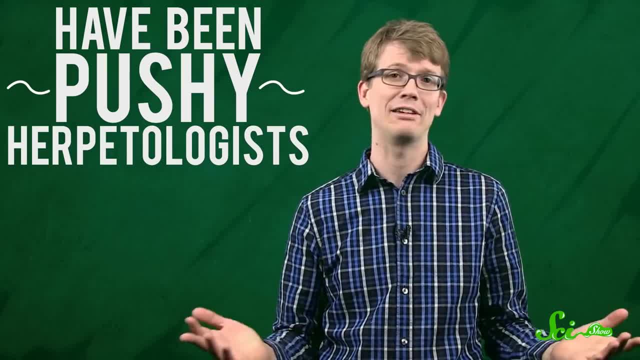 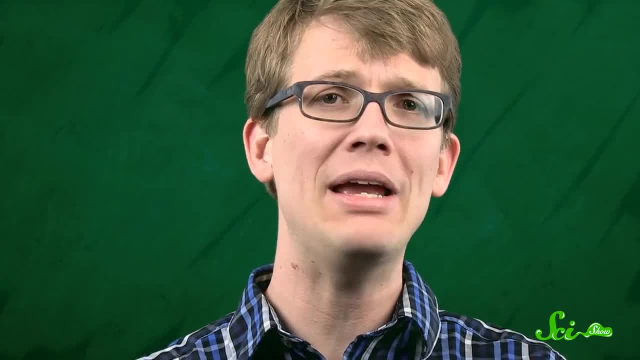 bite victims have been pushy herpetologists who were really kind of asking for it. Relax, they have the antivenom, While the next creature is technically poisonous and not venomous, it's also amazingly potent, so we had to include it. 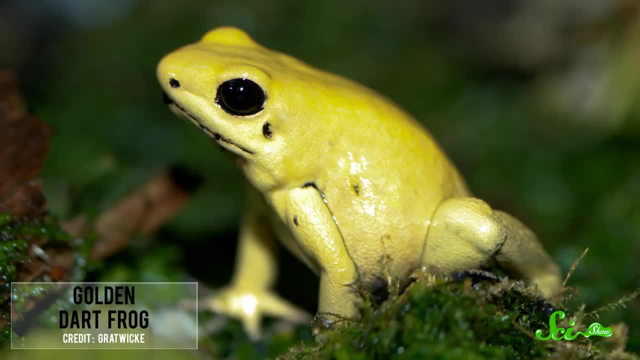 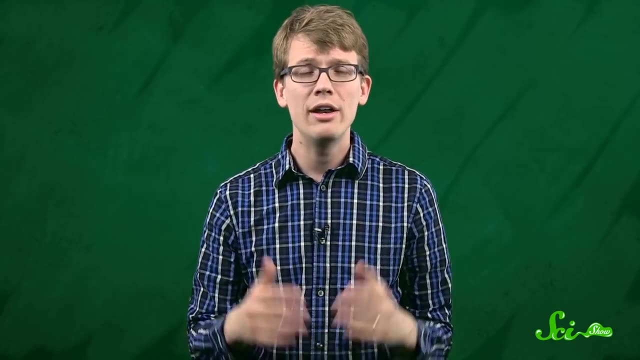 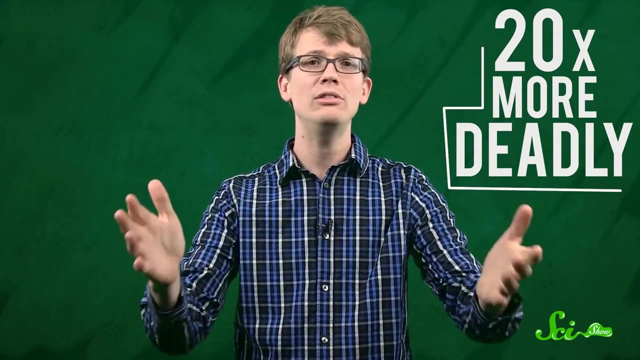 Meet the golden dart frog Found in the Amazonian rainforest. these five-centimeter psychedelically colored frogs secrete the most powerful animal toxin in the world, an extraordinarily poisonous alkaloid called batrachotoxin. It's at least 20 times more deadly than any other poison. 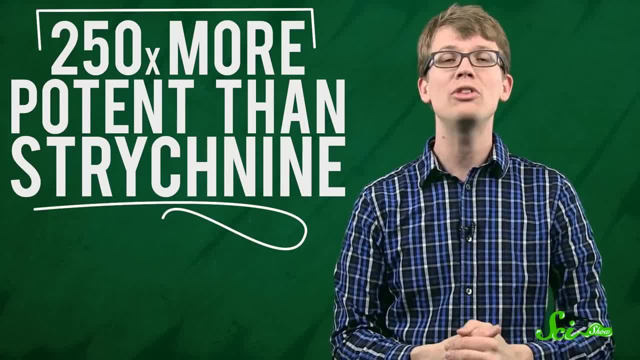 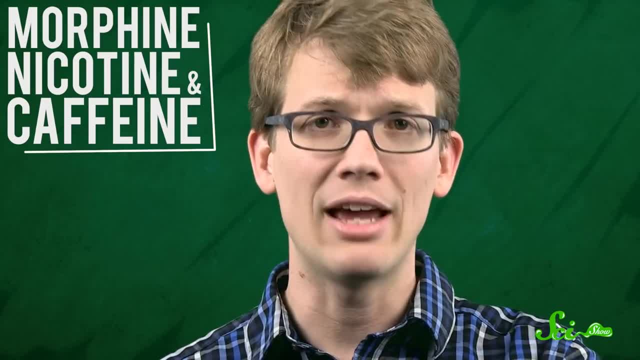 frog species' poison and about 250 times more potent than strychnine. Alkaloids are complex bitter organic bases typically found in certain seed plants, Morphine, nicotine and caffeine- All types of alkaloids that distinctly affect humans who consume them. 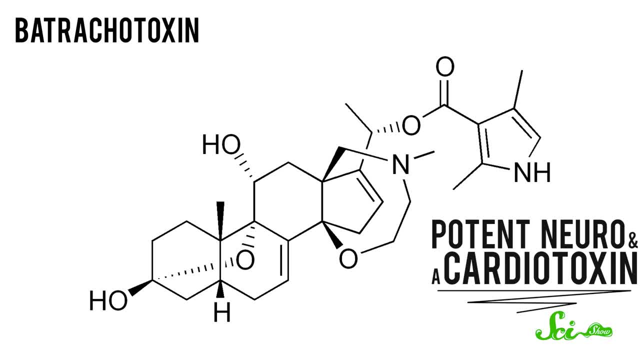 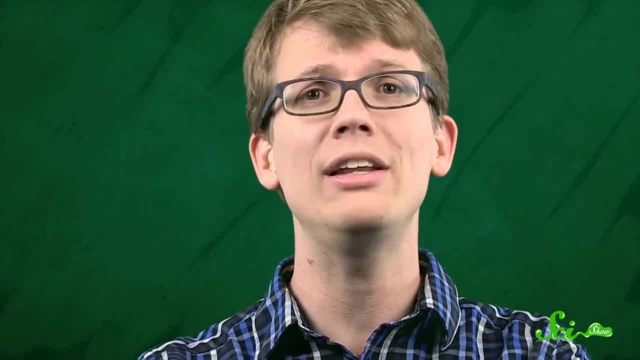 Now, batrachotoxin is an insanely potent neuro- and cardiotoxin, which means it sucker punches you in your brain and in your heart, which are both very important to being alive, quickly stopping the transmission of nerve impulses and leading to near-immediate paralysis of. 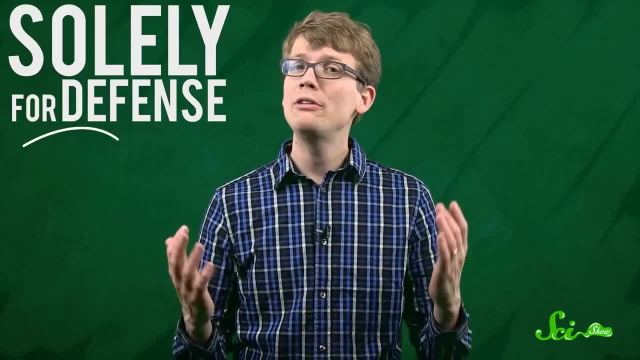 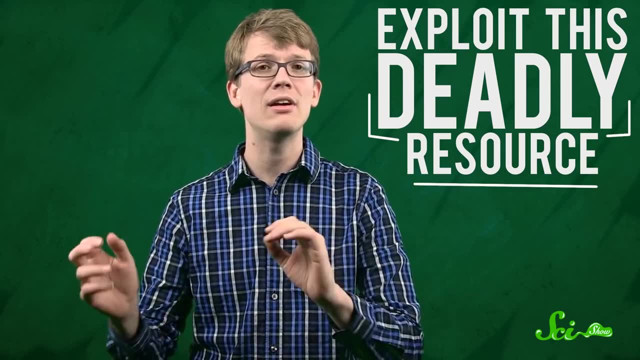 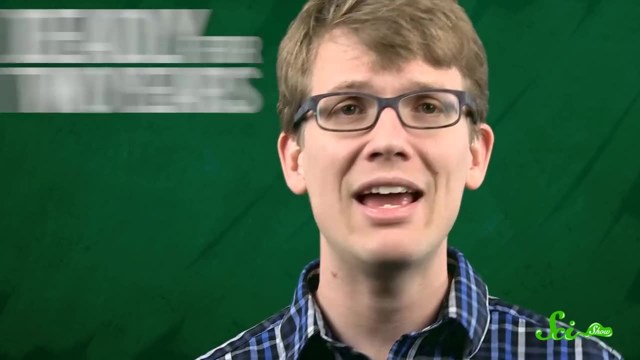 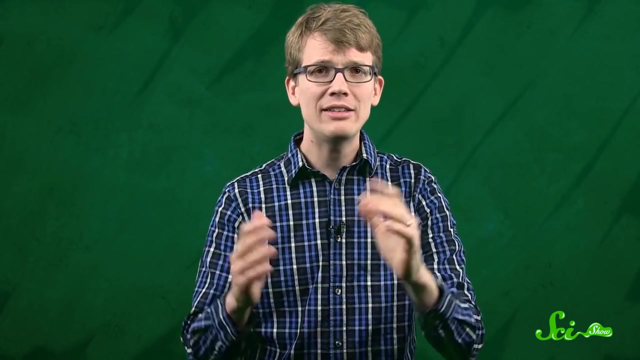 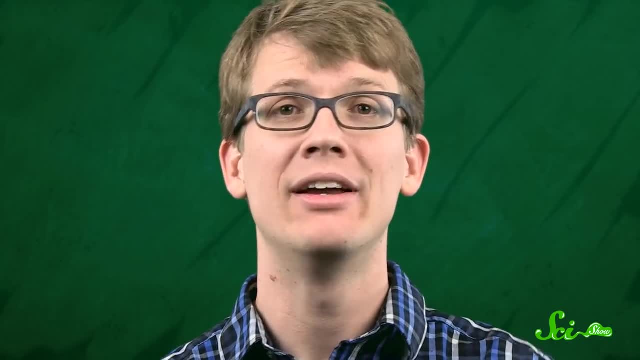 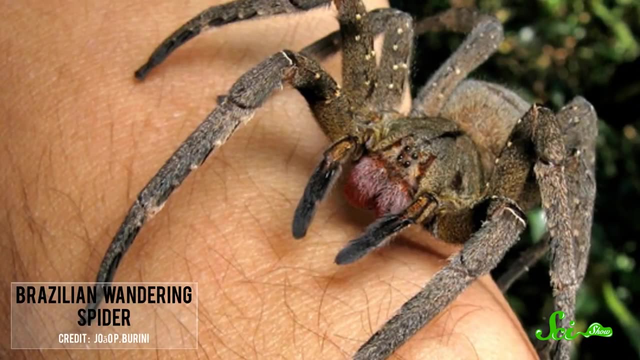 And how could I talk about toxic animals without mentioning a spider? Well, meet their venomous king, the hairy, hand-sized Brazilian Wandering Spider, Called wandering for its tendency to rove around at night. during the day, these guys hike high under logs and in clusters of bananas. They're on a perpetual walkabout, not just in Brazil. In 2005 one turned up in England when it crawled out of a fruit bowl full of imported bananas and bit some poor chap right there in his kitchen. He was fine after a week in the hospital, Unlike many spiders. these guys are pretty aggressive. 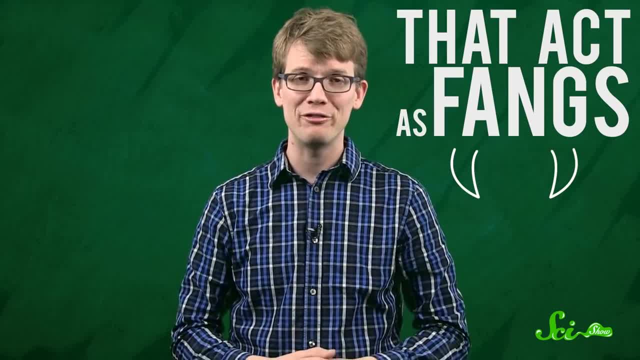 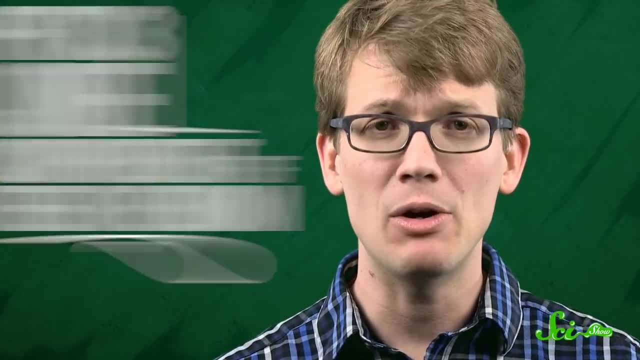 and use modified forelimbs that act as fangs to inject their venom into anyone who honks them off or looks good to eat. The neurotoxin PHTX3 is one component of the venom. It overstimulates serotonin receptor sites on nerves throughout the body, causing intense pain. 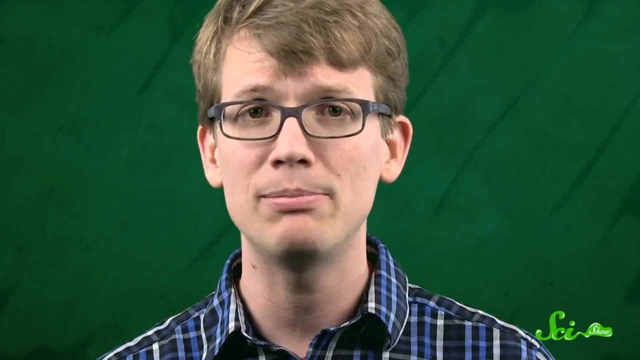 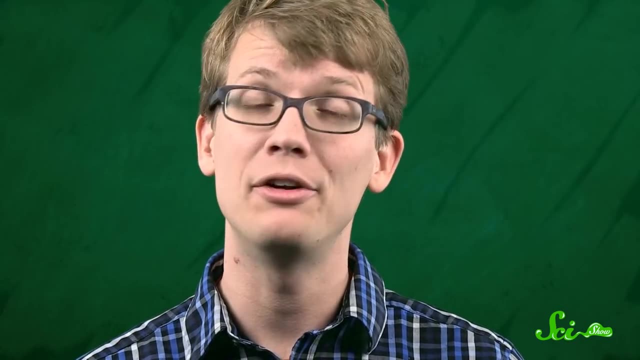 Meanwhile, the juice gets to work on paralyzing your muscles, which can be especially problematic when your diaphragm freezes up, leading to asphyxiation. Luckily, there is an antivenin, if you can find a dose quick enough.